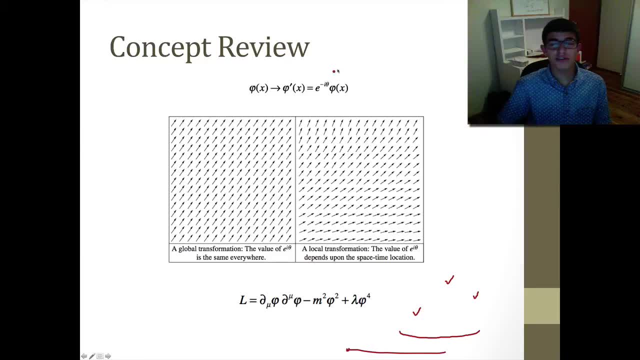 Just a little bit of a concept review. Notice: the theorem states that if you have any symmetry, any continuous symmetry, there's an associated conservation law. So what that basically means is that we can have a transformation under this form and, essentially, the value. 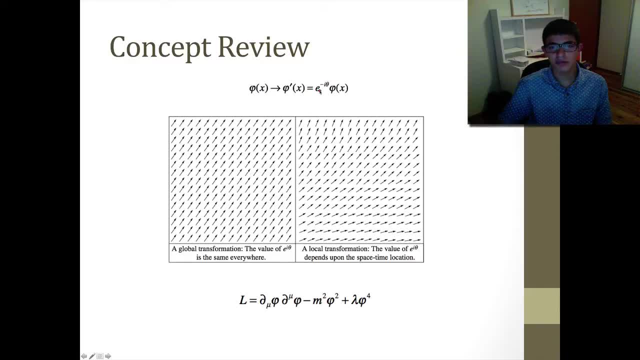 for phi remains essentially the same: e to the i theta. You can think of e to the i theta as a positional unit circle. So the U1 symmetry responsible for electromagnetism is invariant under this transformation. Now there's two types of 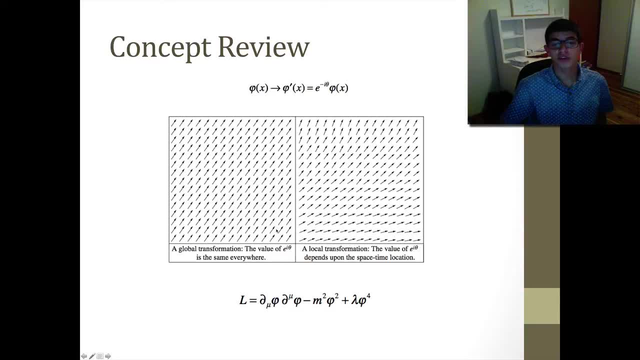 symmetries, really global and local. A global symmetry is where the value of e to the i theta applies everywhere. So if you take any arrow here and I want to look at the value, it's the same everywhere, right? So it's not very. it doesn't depend on its position, Whereas 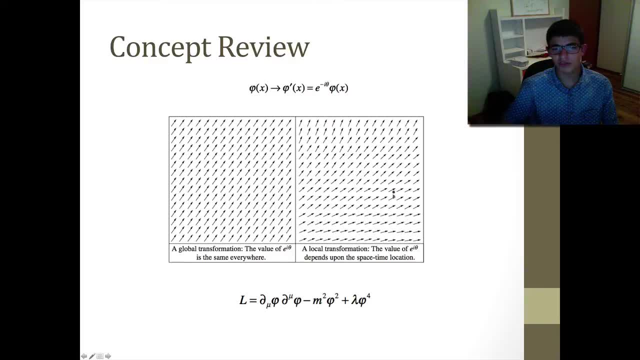 here in a local transformation. each of these arrows has a different value depending on its position. Now to examine the Higgs mechanism- how particles get massed- we're going to be looking at the so-called phi-4 theory. This 4 here represents 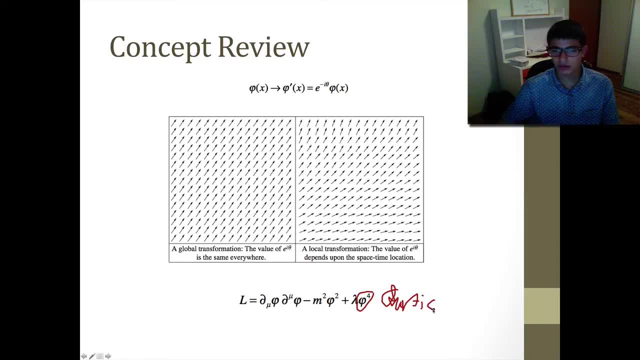 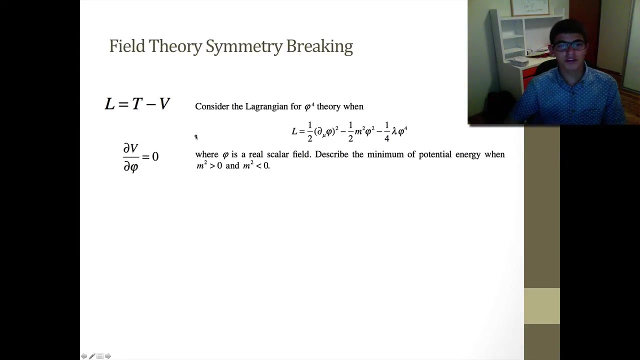 a quartic interaction. We're going to look at a phi-4 theory and how that self-interacting theory and we're going to also look at that Lagrangian and how that generates mass through spontaneous symmetry breaking. So this is the review. So essentially we can imagine the Lagrangian as the final position. 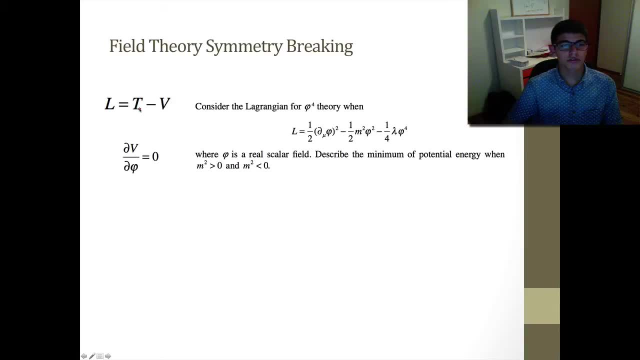 minus the initial position, in other words your kinetic minus your potential energy. and then you've got your- sorry, your potential energy minus your kinetic energy. and then you've got your Lagrangian for the 5-4 theory in the Klein-Gordon form. so this is in the form of the Klein-Gordon equation, right here. 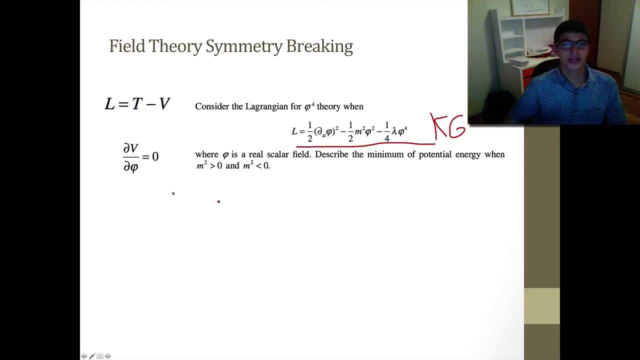 this is the Klein-Gordon form and essentially, to break this symmetry, we need to find the minima. so we need to find the minima of this symmetry, we need to find the minima of potential energy when m squared. essentially, here this term, here this quadratic term. 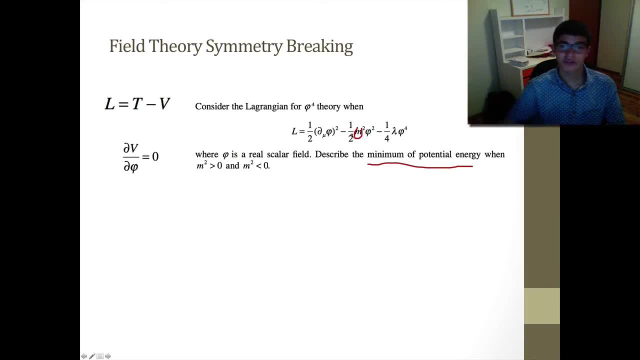 um, essentially, this quadratic term here is more than one, sorry, more than zero and less than zero, and this, by the way, is kinetic energy. this is potential energy. so we're going to look at the minima to find the minima we can use. 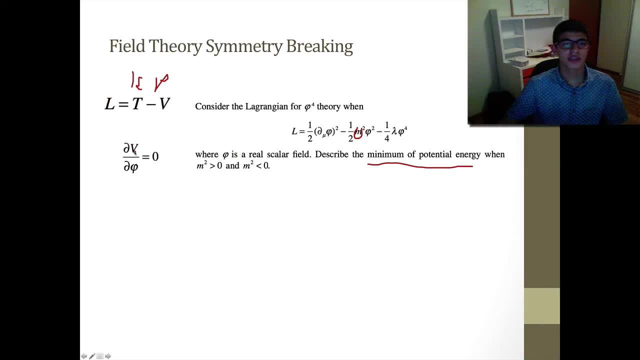 elementary calculus, find the derivative of the potential energy with respect to phi, and we expect to get the minimum term, which in this case should be zero. so how do we solve this? Well, I've written a solution here now, as following this form of the Lagrangian 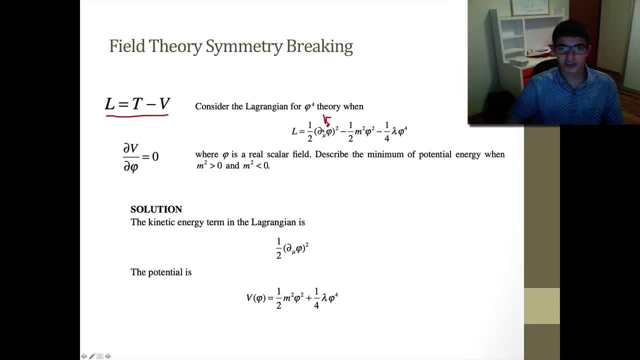 the kinetic energy term is essentially here. this is the kinetic energy term and we've expressed that here. alright, and this is the potential term. the potential energy here is expressed here. this here is your potential term and we've put that down there. so now what we do is: 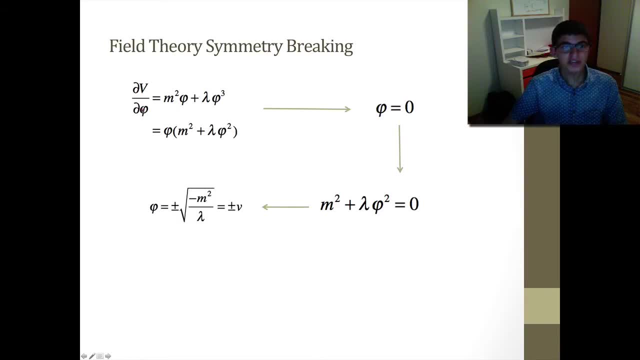 well, we have to compute the derivative and this is a partial derivative. so in a partial derivative there's more than one variable. so this is the result we get from this partial derivative and, as a result, the minima of the potential. at this point, by setting so we obtain the minima, basically by expressing: 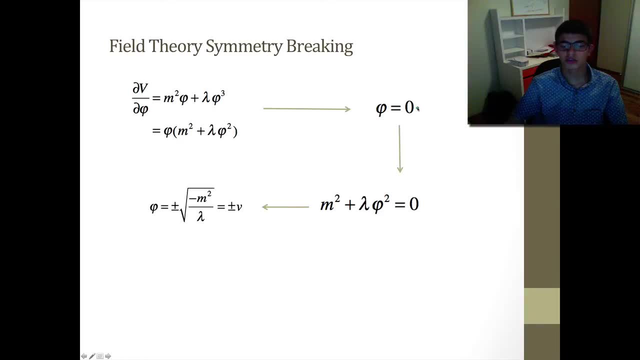 by setting the expression to 0.. Now this of course, corresponds to the case where m squared is more than 0. And we're going to look at how you can actually graph, how you can actually plot the graph or sketch the graph for that. 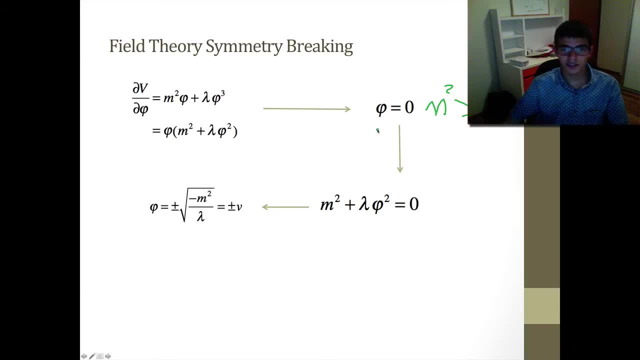 You can think of it as a function. Now, when you differentiate that again, we obtain the second minima. There's actually two minima here, which corresponds to the state where m squared is less than 0. And you can think of this as sort of 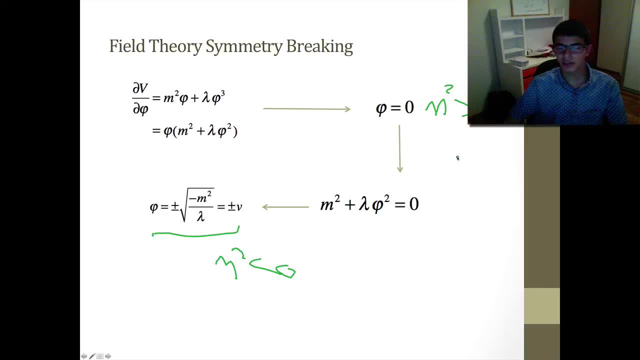 You can think of phi equals 0 as sort of. You can think of it almost like a bowl. Imagine we have a potential in the shape of- almost you can say, a Mexican hat, And on top of that Mexican hat I have a ball. 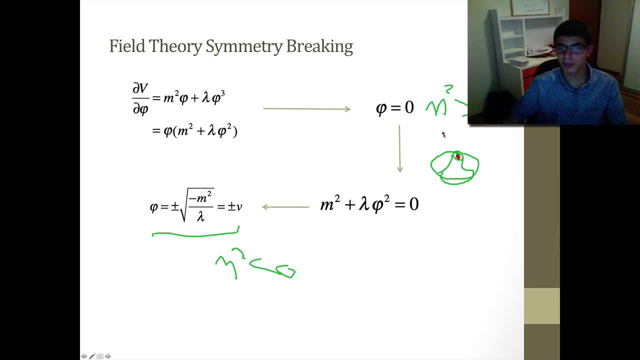 Right, That ball is there on top of the potential. It's in a metastable state. So phi here is equal to 0. That's the metastable state. So this is the symmetry, Now the alternative minimum that we could get. 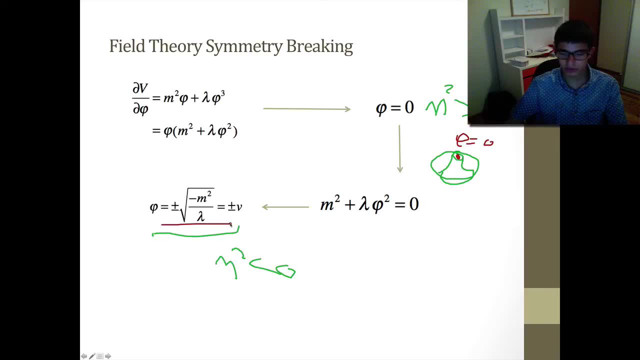 that we just obtained by differentiating was this, So this actually appears as a square. Since it's a square, we have two possible minima: plus or minus. And plus or minus, So phi equals 0,, which is when the marble is on top of the ball. 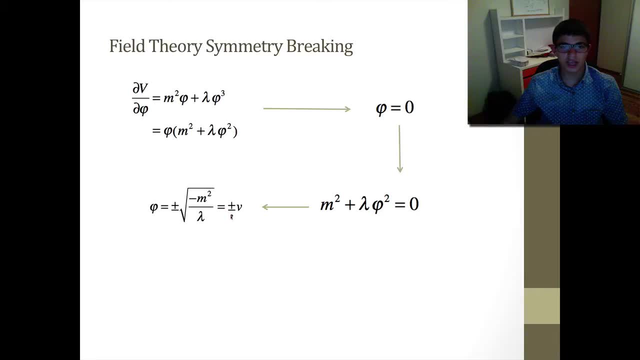 which is when the marble is on top of the ball, and this term here is basically when the symmetry is broken and the ball finally falls. So now we've plotted the point. This corresponds to the case for this here, for phi equals 0,. 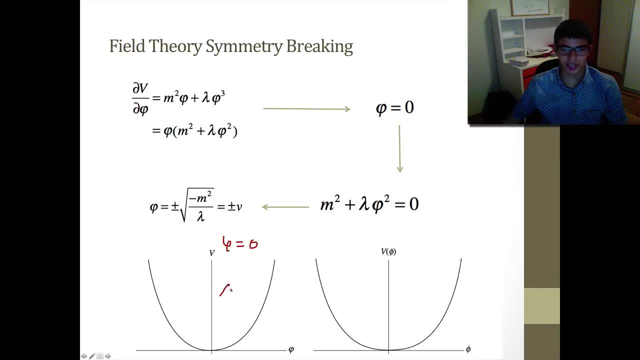 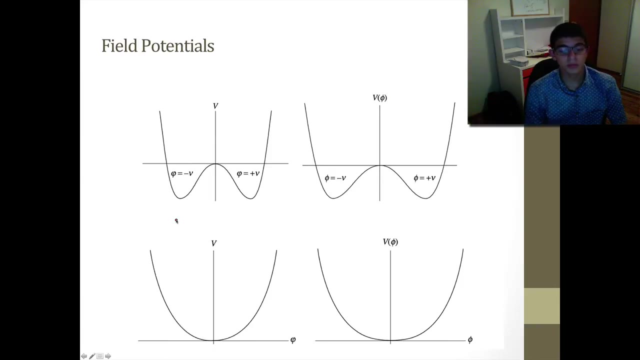 where, essentially, for the case of m, squared is more than 0.. This is how It's a very It's a parabolic sort of curve. Okay, but notice also that when we actually compute this for when m is essentially less than 0,, 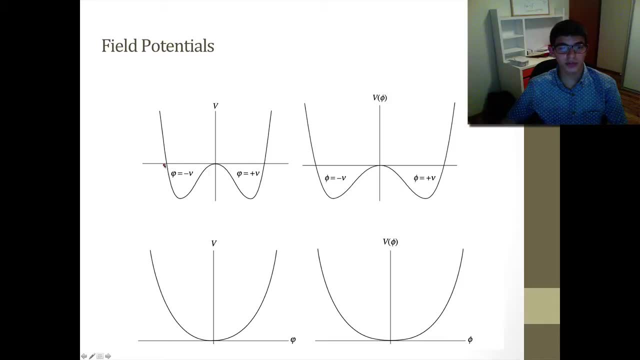 this is the result that we get. We get on the ground state: the symmetry is broken. So this is the very essence of spontaneous symmetry: breaking The lowest energy state or the vacuum state has less symmetry than the resulting interaction. This corresponds to the case where m squared. 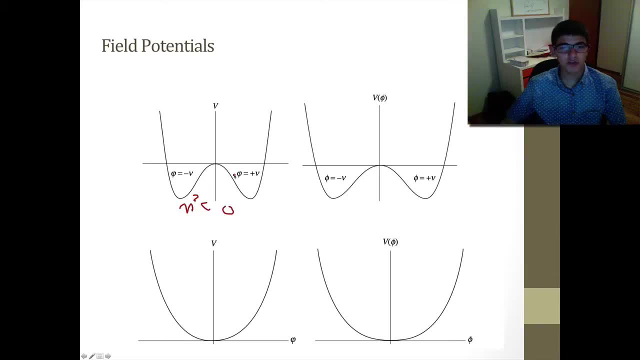 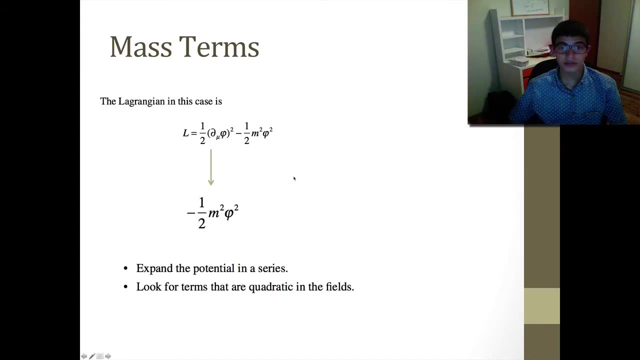 is less than 0.. This is the potential for the Lagrangian. Now the true minimum we want is a plus v, which is right here. So so far, so good. So how do we identify mass terms in the Lagrangian? 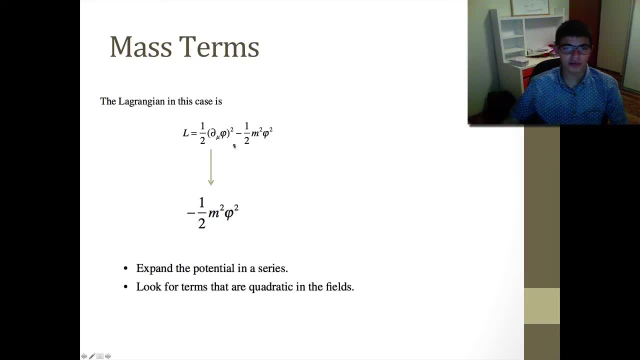 So I've told you that we've expressed this Lagrangian for the 5-4 theory in terms of a Klein-Gordon type. Now, a mass term is always going to appear as such: A minus 1 over half m. squared phi, squared right. 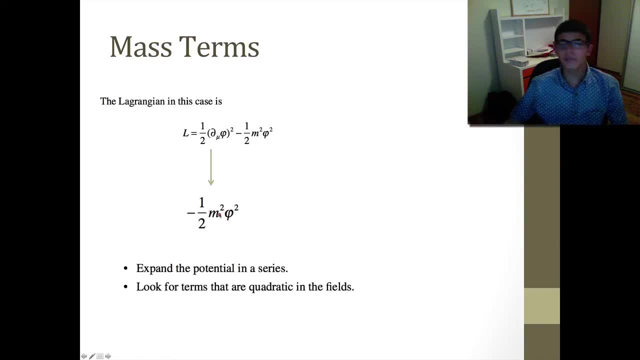 So it's always an m squared, It's always a quadratic term, But sometimes the mass term is hidden. So if the term is hidden, it might look as if the Lagrangian has no mass term, but it may in fact have a mass term. 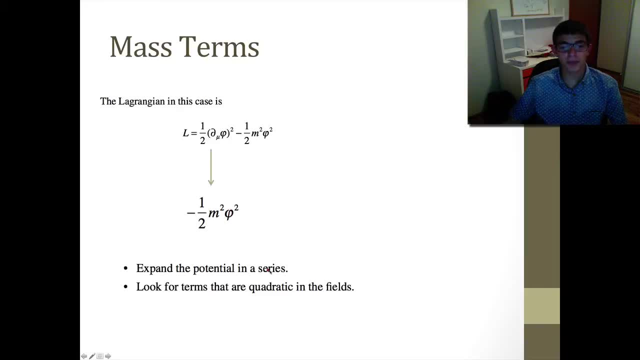 So how do we check for a mass term? We check for a mass term by expanding the potential into a geometric series, or a geometric series or a geometric progression, all right, And then we, essentially- I'm going to show you how to do that- 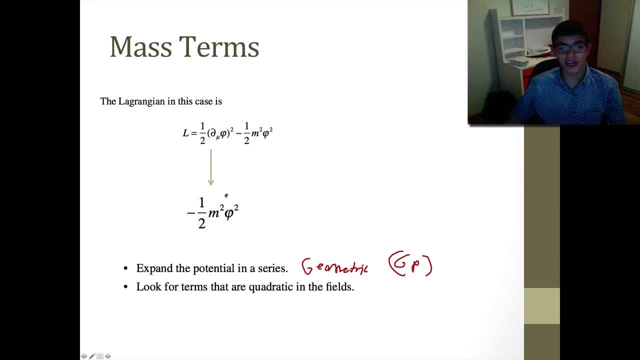 by applying a logarithm. and then we look for terms that are quadratic because, remember, the mass term has to be quadratic. So how do we do that? Let's take this term here, okay, And this term here, this Lagrangian. 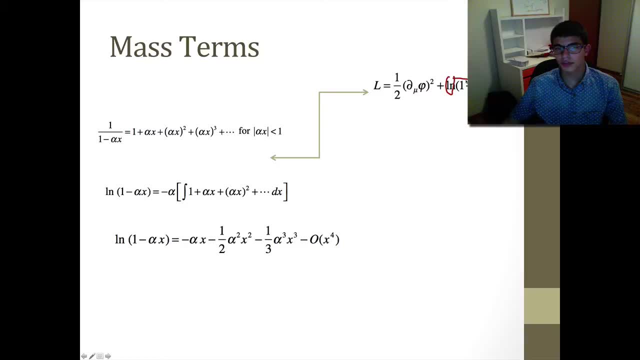 has a natural logarithm multiplied out by this. So let's expand that out. If we expand that out as a geometric series, it's essentially 1 plus an infinite amount of terms, And remember that AX is always less than 1.. And simply we can expand that out. 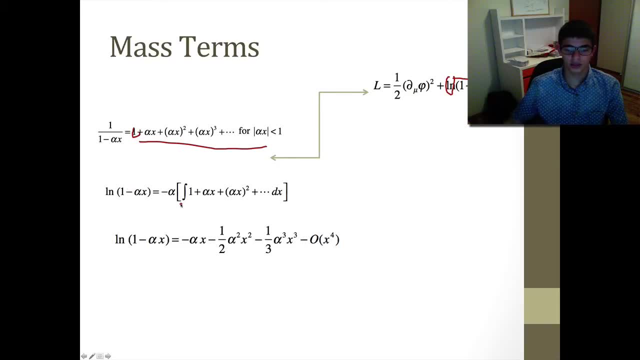 And what we've got to do is introduce a logarithm into the expression and we simply bring the minus A outside the series, outside the integral, and we just integrate all the parts, And then we see, after we obtain the result, that, yes, indeed, we do have a quadratic term. 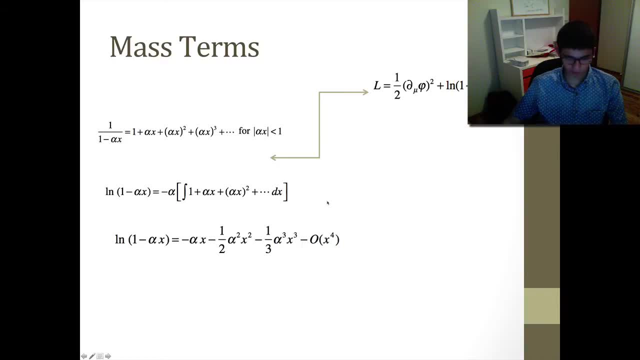 which is a minus 1 half. It's right here. So this Lagrangian here at first looks like it doesn't actually have a mass term, It just has a natural logarithm. But when you actually do the geometric series, 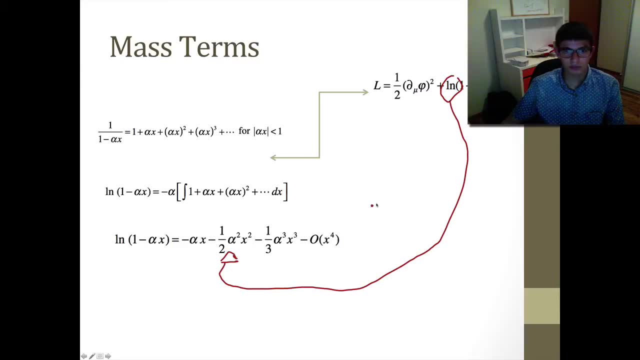 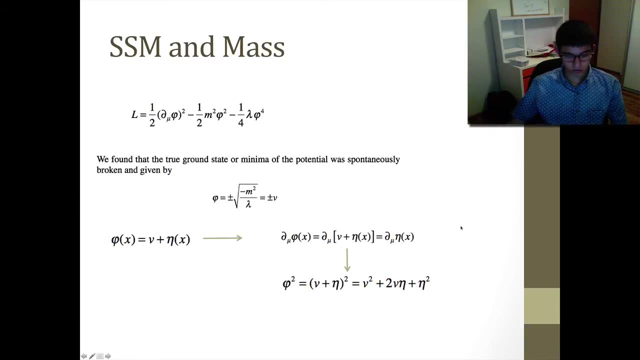 it does actually have a mass term. Okay, so now let's look over spontaneous symmetry breaking. So what we've got to do now is that we've actually so, as I've written here, we've found the minima as such, at plus or minus the root of negative m, squared over lambda. 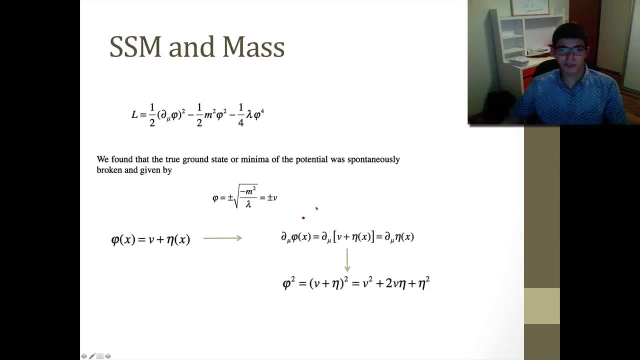 which equals plus or minus v, which was the 2 minima that we obtained. Now what we're going to do is we are going to essentially spontaneously break this symmetry. So what we're going to do is we have to write the fluctuations around phi. 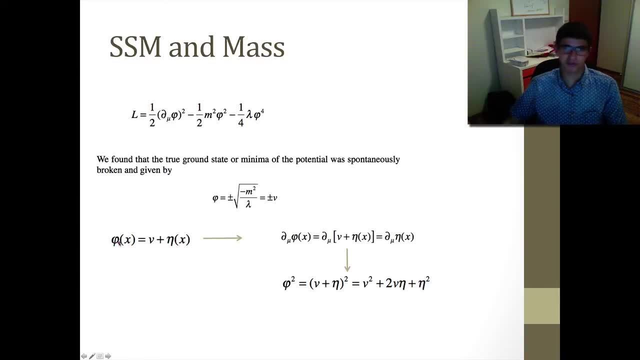 We can imagine. since we're doing quantum field theory, imagine phi as a field. All we have to do is express the fluctuations of phi about the right-handed minimum, which is v or positive v, And then we just add this extra eta term. 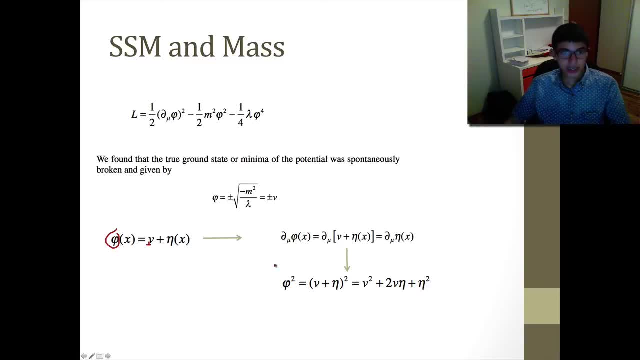 which is here It looks like a funny-looking n. So expanding that out into the Lagrangian, we essentially get our phi as v plus eta to the x and essentially equaling partial derivative mu eta x. And then if we square that to get a quadratic term. 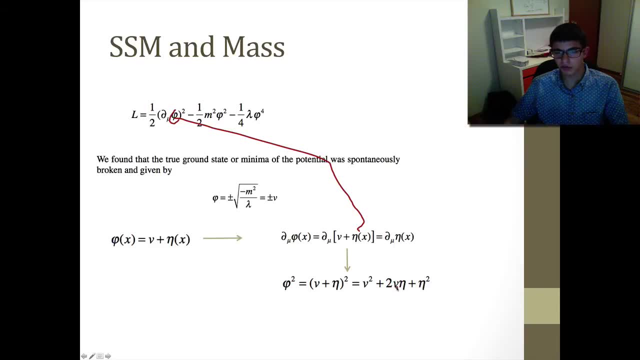 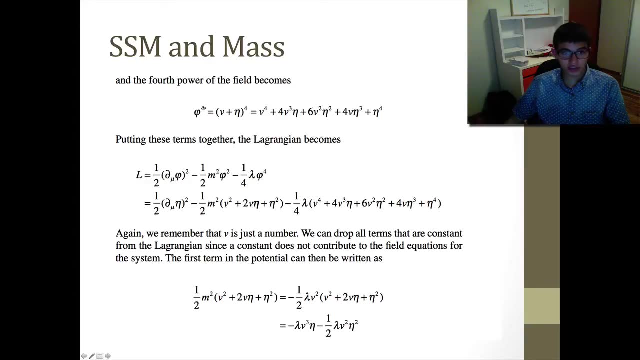 we're just using the binomial rule, We get v squared plus 2, v eta plus eta squared, And if we expand it again, we start to get the phi 4 theory. We get this expression here, But let's put these terms together. 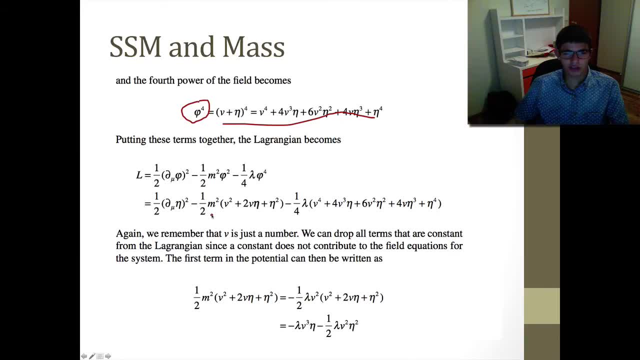 Putting the terms together, we get this very long Lagrangian. But I've written here that you have to remember that v here is just a number. I'm not sure if it's a v or a mu. Let's call it a v for now. 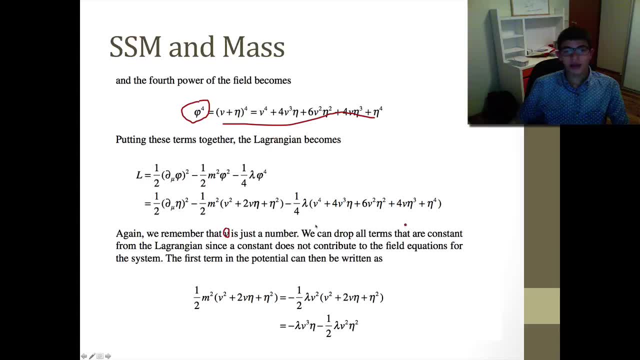 So, since it's just a number, it's just a constant. basically It's not a variable, And what we know from field theory, if you're familiar with it, is that constant terms don't actually contribute to the dynamics of the field equation. 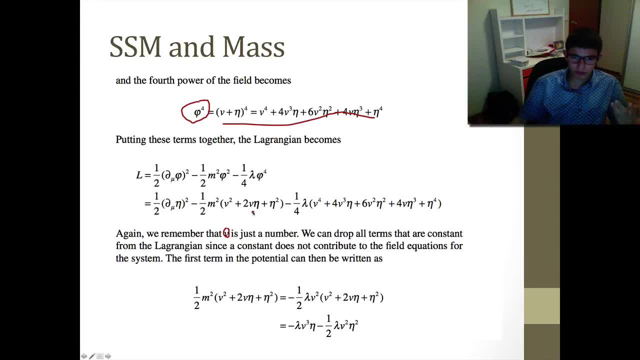 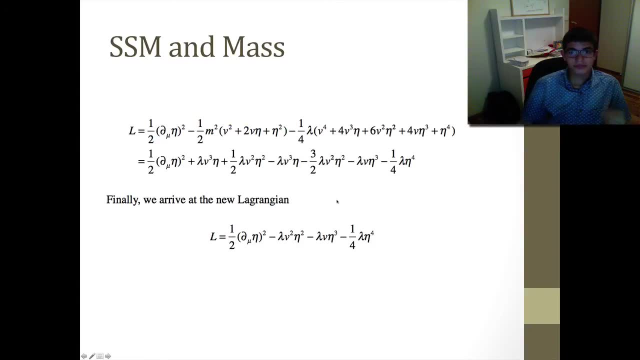 So we can simply drop them. Dropping the constant term v, you simply get this result here. It simplifies to that. And then again, if you put back what we obtained before here, if you put all of that together, 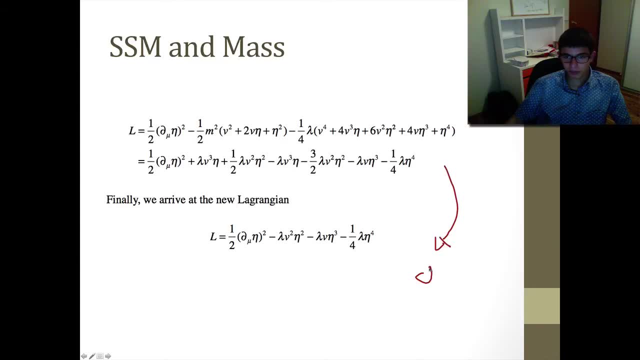 and then dropping the constant term, dropping mu constant- and we arrive at this Lagrangian. Okay, So we've arrived at this Lagrangian. Now, what does this Lagrangian actually mean? What do all these funny-looking symbols mean? 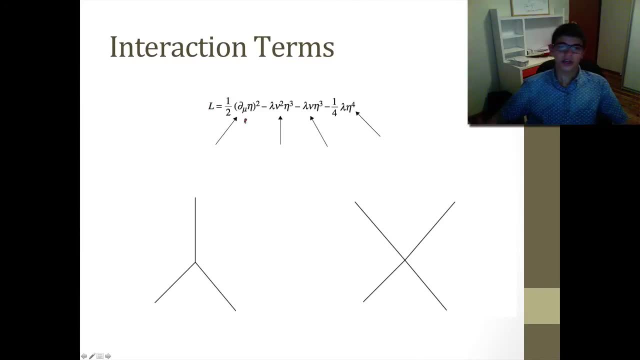 Surely there has to be some sort of mathematical meaning. So let's look at the first term. We already discussed this term here is kinetic energy. This, of course, is a quadratic term, So this must be the mass term. This here is a self-interaction term. 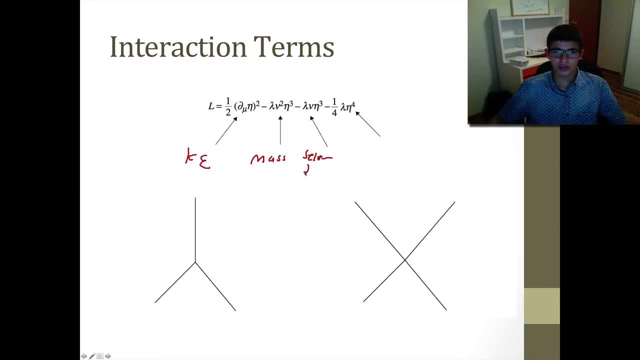 And I'll show you what that means in just a minute. Self-interaction, self-interaction, Right, But okay, So self-interaction. This is a cubic self-interaction, So that corresponds to three legs: One, two, three. 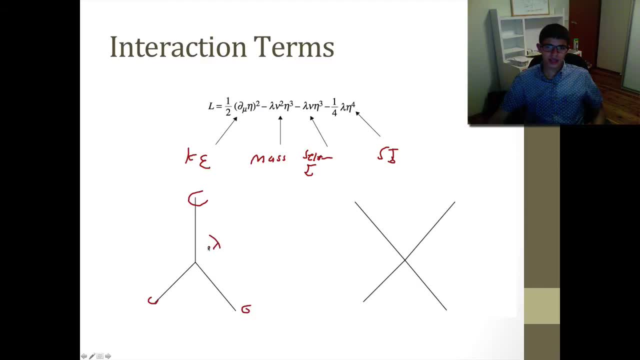 This Feynman diagram here represents the negative lambda mu squared self-interaction. This here is a quintic self-interaction, So it's two of four. So there's four interaction legs: One, two, three, four. This represents the case one over four. lambda eta to the fourth. 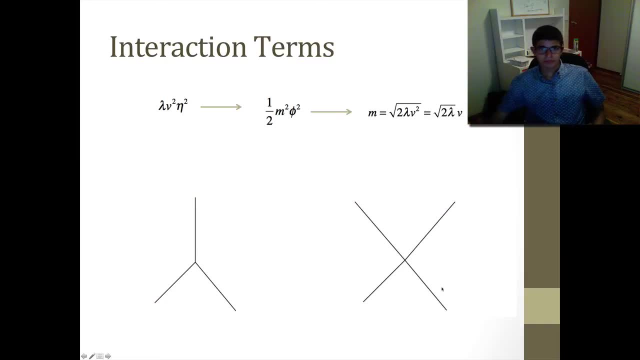 These are our self-interaction diagrams And essentially we can extrapolate this result to obtain the mass. We obtain the mass as such And since the Klein-Gordon Lagrangian says that the mass term has to appear in this sort of formalism, 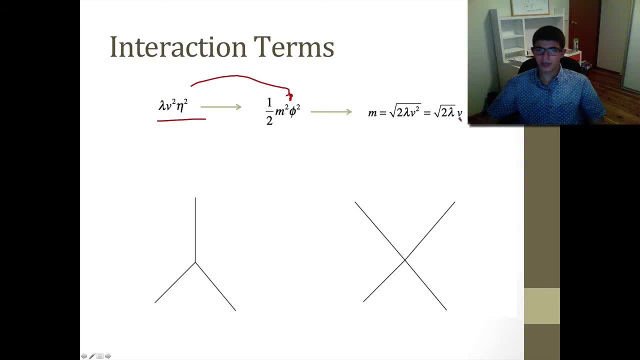 we obtain the mass as root, two lambda mu And again the self-interaction terms. Okay, So so far we've only considered one particle. In most physical situations and scenarios there's more than one particle produced in the symmetry breaking. 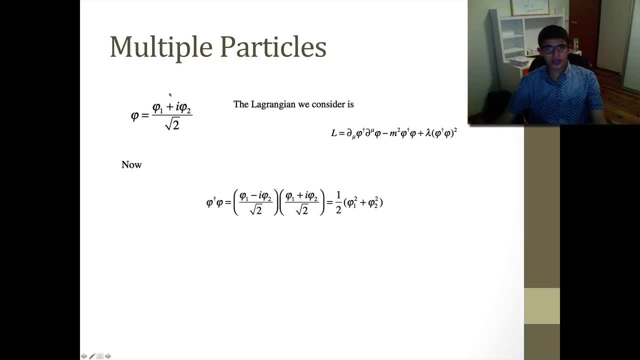 So, like your lecture on the lecture week theory very similar. We're going to again break up the field into two components, two scalar components, And we're going to consider this Lagrangian here, And then we have phi dagger as equaling. 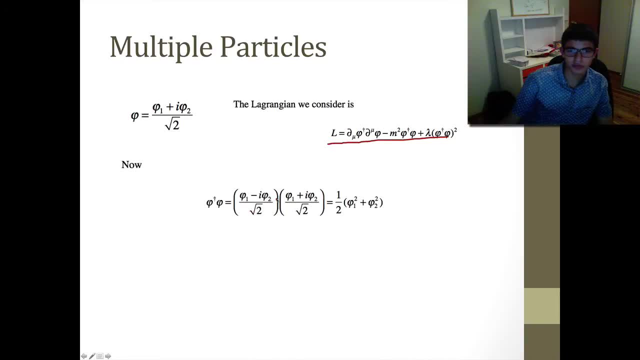 This is equaling phi one minus i, phi two over root two. The only difference is the plus and minus sign, because it's a complex conjugate. So essentially, when you expand that out, you get this result here, And this is similar to the Klein-Gordon type, except that the quadratic term is split into two other quadratic terms. 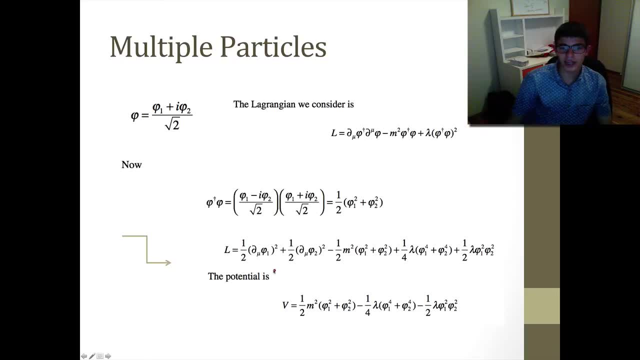 Okay, So multiplying out, we then obtain a potential. Remember that The kinetic energy minus the potential energy in the Lagrangian. So if we forget about this for now, This is just our kinetic term. That's irrelevant. What we're interested in is this term here. 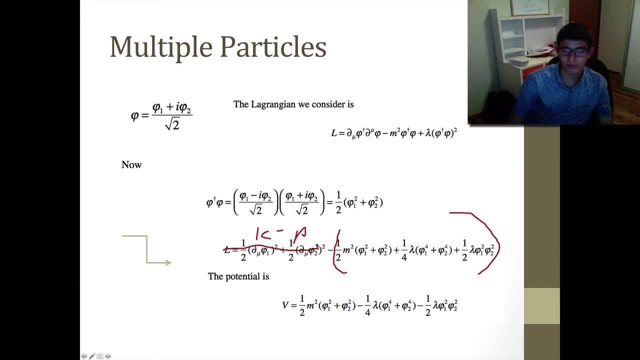 This term onwards. This is our potential term. Remember the Lagrangian Kinetic energy minus potential energy. This is our kinetic term. That's our potential term. That's the potential. Okay, We can also. I'm going to do a lecture on group theory. 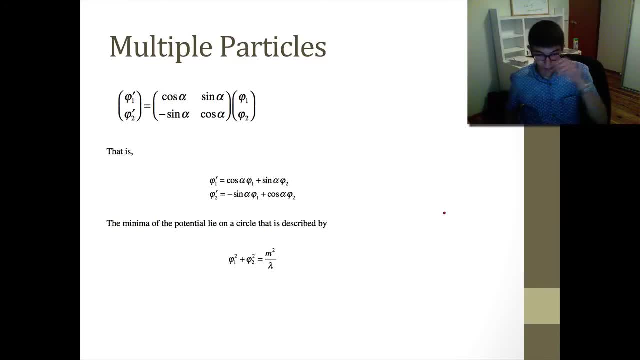 But if you're interested in group theory, we can express this in terms of rotations in the phi prime one, phi prime two space, And you can, you know. So these are essentially rotations. So phi prime one equals cos alpha phi one plus sin alpha phi two. 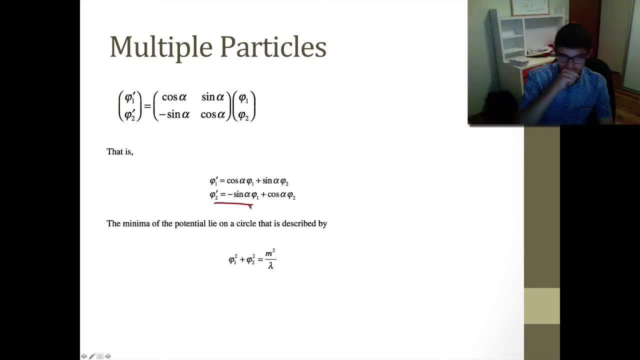 Just multiply that, You get pretty much a similar answer for phi, prime two. And again, the minima lies on m squared On m squared over lambda For these two components of the field. So the minima So we need to express: 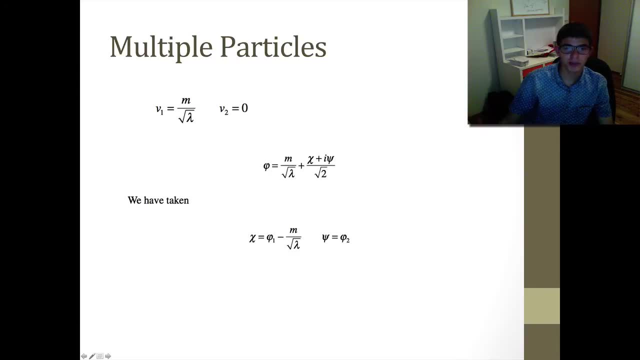 Okay, So there's two minima, like we discussed. There's phi equals zero, And then the other minima that we get from differentiating again. So what we want to do is we want to express the two minima again. 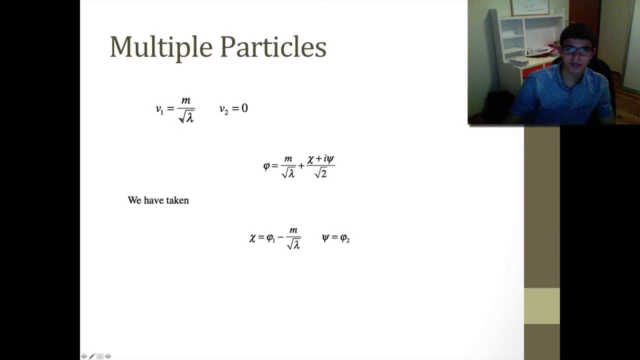 So since we expressed phi in terms of two components, Let's express phi in terms of v one plus v two, And then that simplifies to that And just remember. So if you're interested in group theory, This is our potential term. 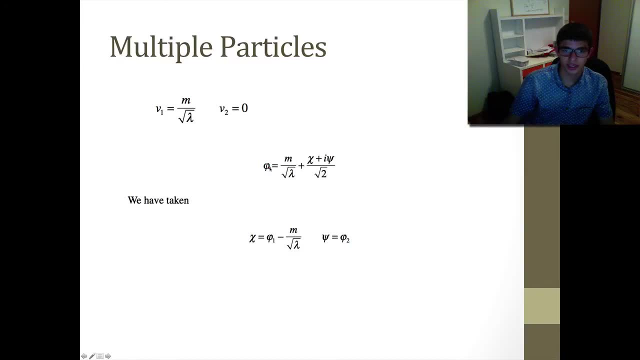 Remember the Lagrangian? This is our potential term. This is our potential term. So if you're interested in group theory, This is our potential term. Just multiply that. Let's express phi in terms of v one plus v two. 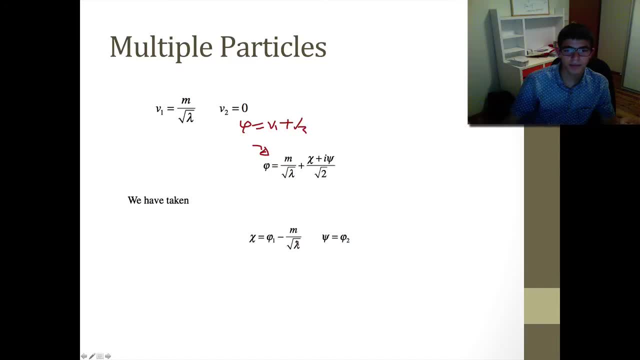 And then that simplifies to that. And just remember that this x, this chi term, or rather it's a Greek letter, chi Is phi one minus m over lambda And psi here, which we represented as a spinner previously, Now we're just using it as a represent. a field is essentially phi two. 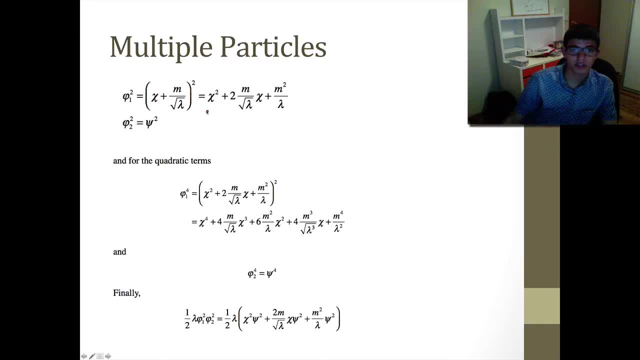 Again, If you square to create a quadratic term, again using the binomial rule, We're getting that as such. For the first double, the product square. the last And pretty much for the psi, we just square it And again, we square again to get a fourth power and we get that result. 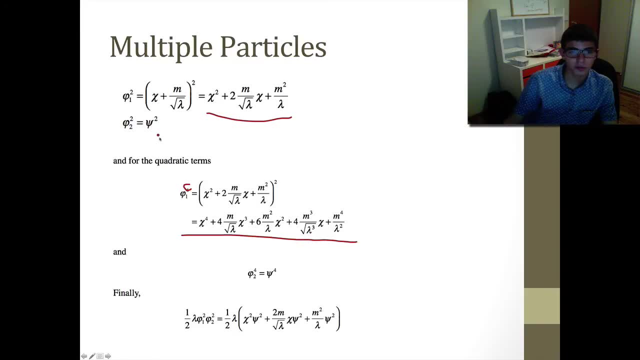 And again to have the psi to the fourth. you square it again and get the side of the fourth And finally, the Lagrangian you get is this: This is a- I believe, this is your, your, your, the term, this is the term that you get as as a result, 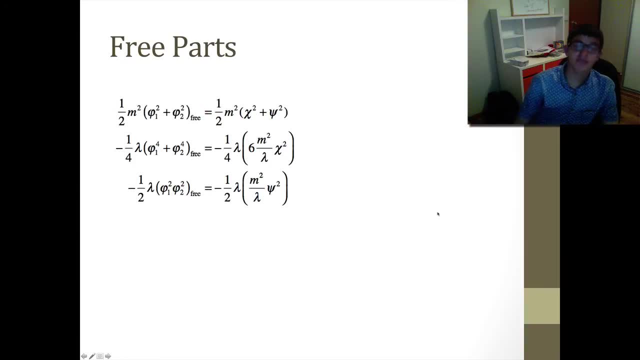 This is a multiple particles. Now, as we said, constants don't contribute whatsoever to the field equation. So dropping the constants from this equation, we obtain the free parts of the of the potential of the Lagrangian. So just drop in the terms: these are the free part, the free parts, not not free, but free. 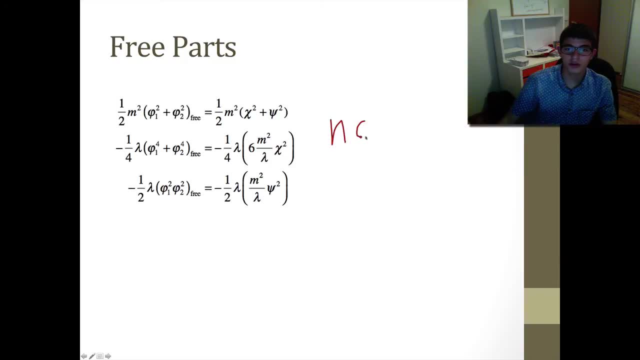 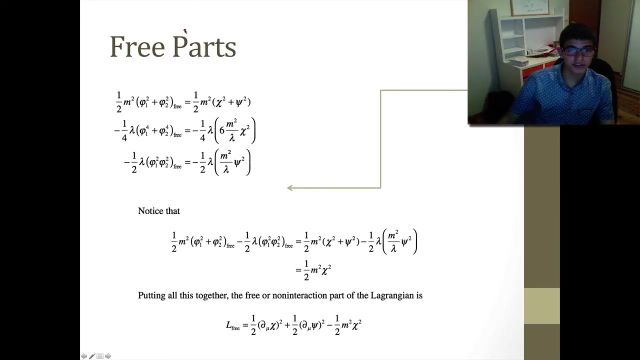 as in emancipated. So free parts- No Constants- Need to get a better pen, Anyway- no constants. So if you notice that if you put all of these together, um, we actually get. if you put all of these free terms together, we get the free part of the Lagrangian. 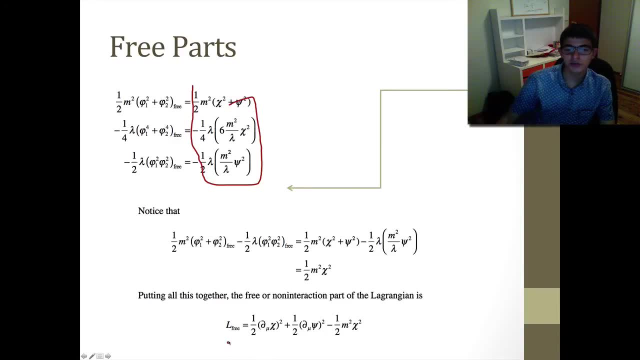 And this is this part of the Lagrangian does not interact. So putting this all together, we get this resulting free Lagrangian. So and if you want to look at, let's look for a mass term: Essentially, our mass term is our mass term is our essentially here, our minus one over. 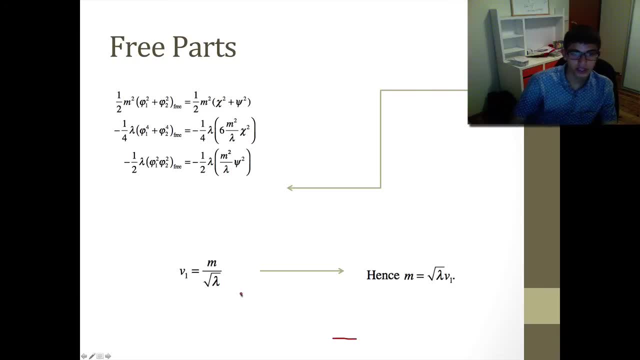 two m squared, eta squared And essentially, since we set v1 as m over root lambda, the mass becomes m over lambda, v1.. Because remember that was a squared term And remember that we set eta to v1, if you remember, Uh okay. 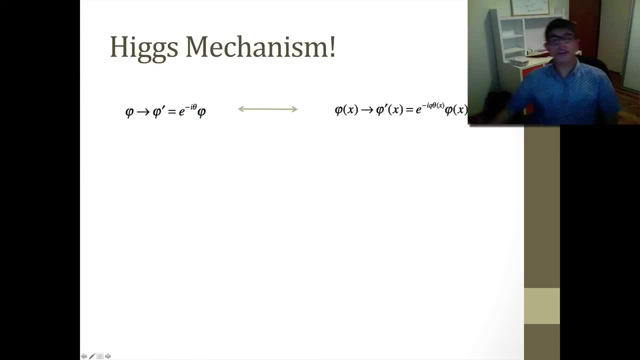 So let's just wrap up the lecture. I want to look at the Higgs mechanism um itself. So recall that under a U1 symmetry, a unitary one symmetry- okay, Lagrangian- is invariant under this transformation. And remember that theta is just a function of space-time. 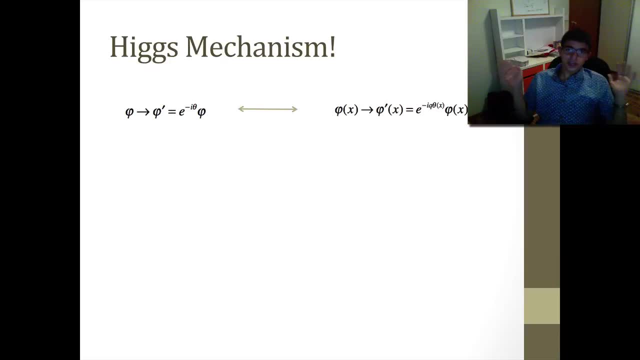 But remember, In the previous cases we considered a global symmetry, But what we want is for a gauge field, is to introduce a local symmetry. So no more global symmetries. From now on, we're going to use no more global symmetries. 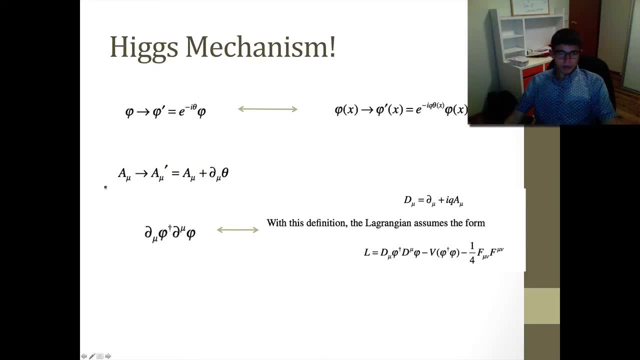 From now on we're going to use uh local symmetries. Remember that in classical uh electrodynamics, if you imagine the field A mu and then perform a transformation on A mu, So A mu prime, This is essentially the outcome. 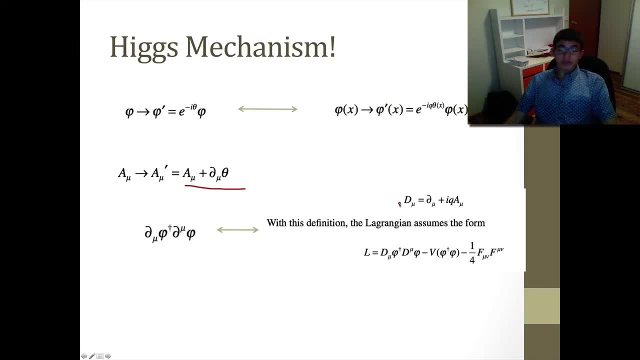 And remember we have to keep the theory covariant, so we have to introduce a gauge covariant derivative. This is very similar to classical electrodynamics with the A mu, Simply d mu is your partial derivative, mu plus iq, A mu, essentially incorporating this. 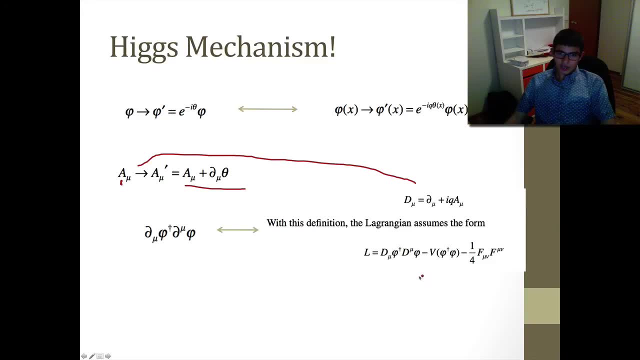 field here. So we're going to have our Lagrangian now, We're going to have our kinetic potent- our Lagrangian equals kinetic minus potential. This here is a kinetic term, This here is a potential. And remember this F mu nu term here is with the subscript: mu nu is the electromagnetic. 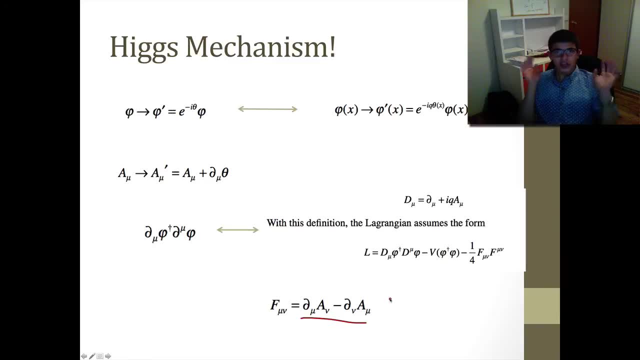 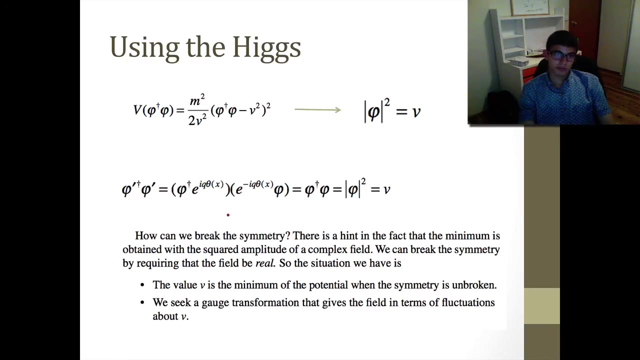 tensor And this is given by this, So it's very much analogous to. so the Higgs mechanism itself is basically the Maxwell type theory, combined with spontaneous symmetry breaking. So now, um, we have to, we want, we want to, uh, we want, we want to break the, um, the. 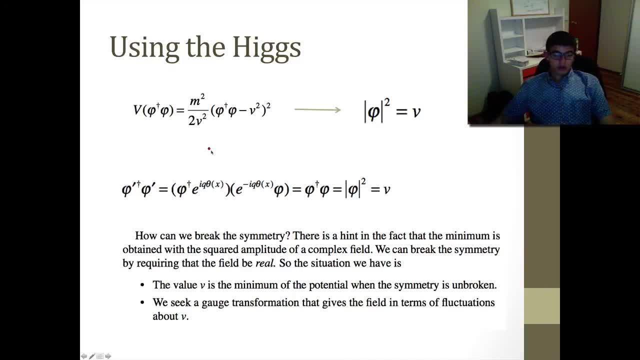 we want to break the symmetry. So what we've got to do is we have to. we've included a constant v squared, and what we have is we've obtained a minimum of uh, of essentially phi squared, to equal that constant. 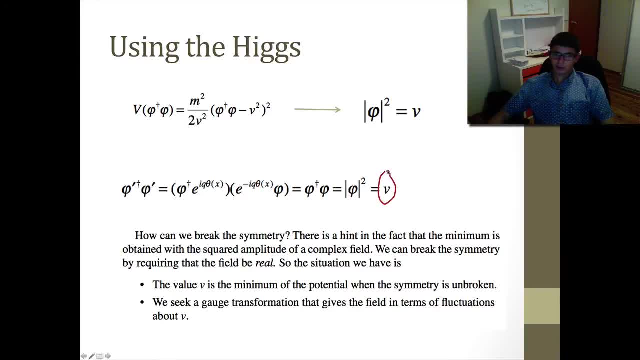 So, simply, we can perform a gauge transformation, we're still going to get the same constant. That's why it's a constant. So I've written a little note here. how can we break the symmetry? So there's a hint In that the minimum is obtained with the square amplitude of a complex field. 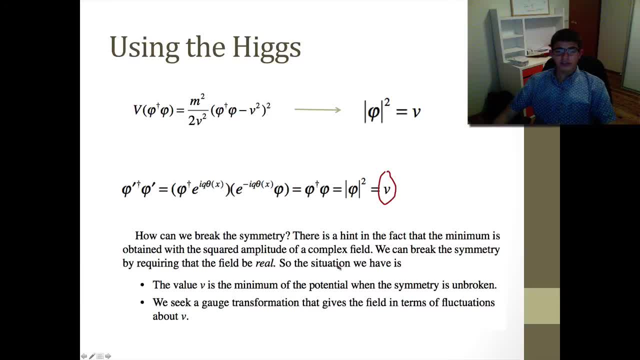 We can break the symmetry by requiring the field to be real. So this is the situation we have: is the value v is the minimum of the potential when the symmetry is broken and we seek a gauge transformation that gives the field in some of the fluctuations. 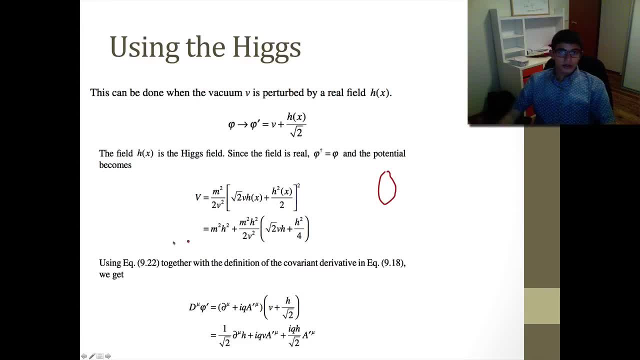 about v. Let's see what that means in a minute. So now what we've got to do is we have to perturb the vacuum. we have to disturb the vacuum using a real field. this is the Higgs field. here hx right, and we're going to. 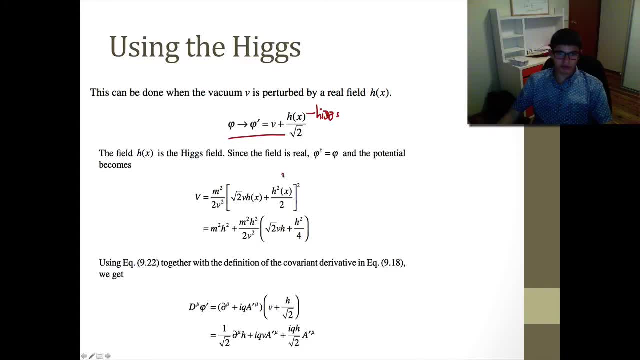 express it as v, Our constant, Our constant, plus hx over root 2.. Simply incorporate that into the kinetic part of the Lagrangian expanding out and essentially what we should get is a essentially this: multiply the covariant derivative by the field. 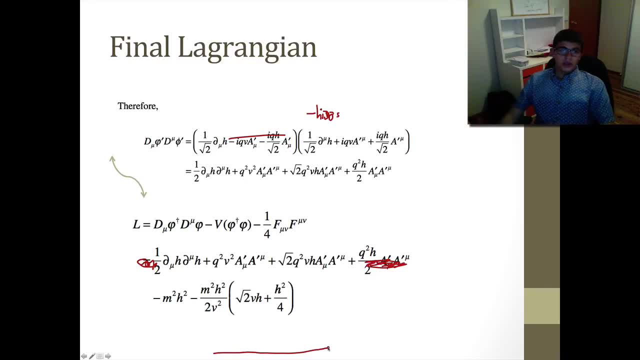 we get this result here. Okay, so what is the final Lagrangian that represents the Higgs field. So in this transformation- this is what we've done- We've multiplied out the covariant derivative, so essentially we've expanded out the kinetic.